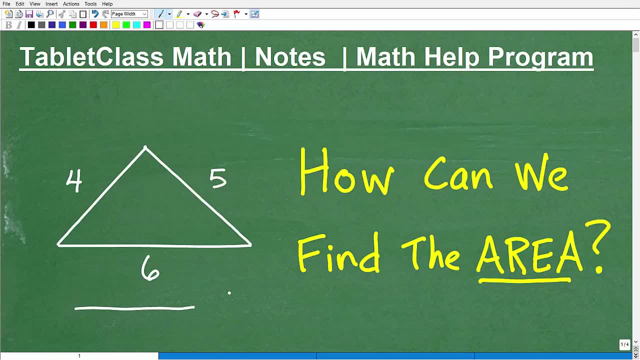 Okay, so we have this triangle here and we want to find the area of that triangle. Now it seems at first glance it's maybe not a difficult math problem. You're like: oh yeah, that's easy. I found the area of triangles before And you're probably thinking to yourself: I need that formula. area equals one half base times height, And that's pretty good thinking. Okay, so if you were like saying to yourself: you're like, you actually remember this formula, that's pretty good. 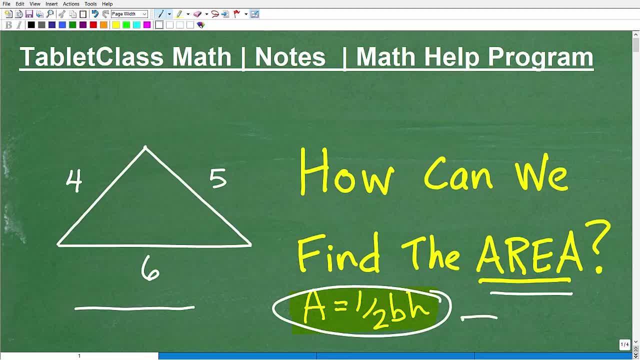 That's very good. However, unfortunately, it's not going to be so easy to apply this formula in this problem, So we're going to need another approach. You could use this formula, but in order to use it, we're going to need some advanced mathematics to help us out, And there's another, better approach to actually calculate the area of this triangle with this kind of information. So stick around here for a couple minutes. I'm going to show you exactly what that formula is and how to use it. 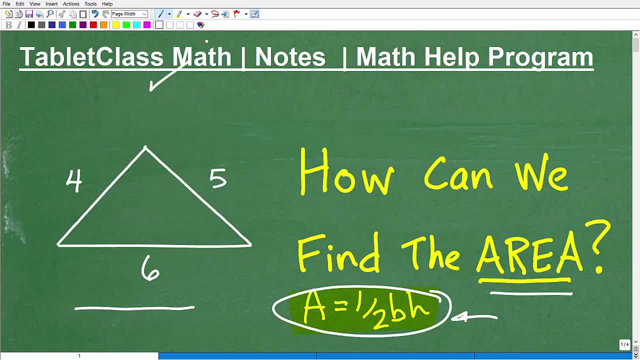 But first let me quickly introduce myself. My name is John. I'm the founder of Tablet Class Math. I'm also a middle and high school math teacher And over several years I've constructed what I like to believe is one of the best online math help programs there is. Of course, I'll let you be the judge of that. If you're interested. you can check out my math help program by following the link in the description of this video. But basically I have 100 plus different math courses, ranging from pre-algebra, algebra one, geometry, algebra two. I'm going to be launching. 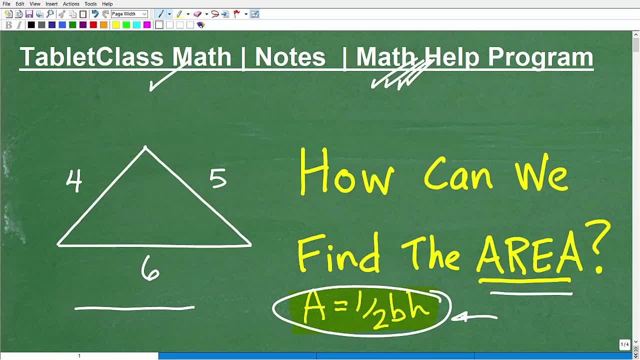 pre-calculus here very shortly. But I also do a lot in the area of test preparation. So if you're studying for like the GED, SAT, ACT, GRE, GMAT, ASVAB, ACCUPLACER, CLEP exam, Let's see here. What other exams am I missing? Maybe a teacher certification exam like the Praxis, or CBEST or CSET, or nursing entrance exam like the TEAS. There's a ton of different exams out there that have a lot of math on it And 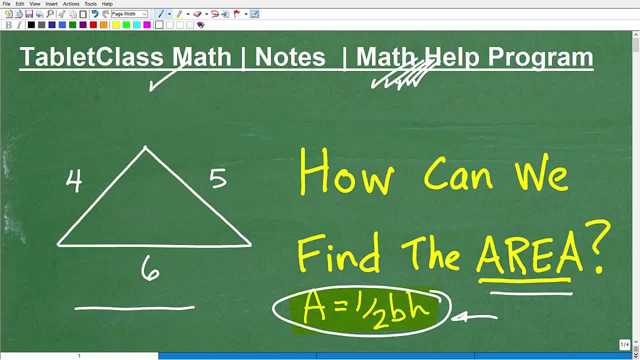 if you don't do well on the math section on these exams, you don't do well on the exam, So that's not a good situation. So if you need help with your test preparation, just go to my website, check out my full course catalog. I should have what you're studying. If I do not, drop me a line and I'll help you out the best I can. Also, I do a lot with independent learners like homeschoolers. I actually have a great homeschool learning system, So if you homeschool, you might want to check that out, And then, obviously, I help those of you that are 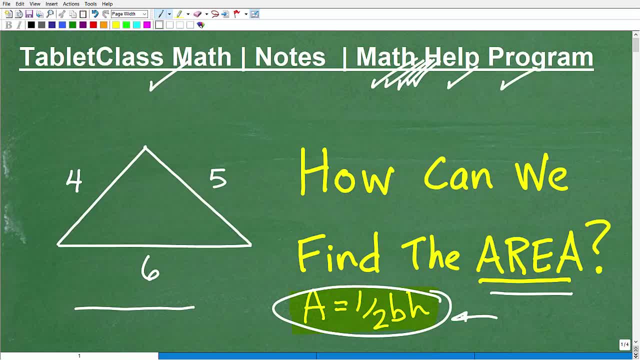 struggling or having a difficult time in your current math courses. Now, the one thing, if you are serious about improving in mathematics, that you got to do for yourself. no one could do this for you. That is no taking Okay. so over decades of teaching mathematics, it's just crystal clear to me those students who take excellent math notes okay, almost always do very, very well in their class. And then the reverse is true: Those students who are like me way back in the good old 1980s- 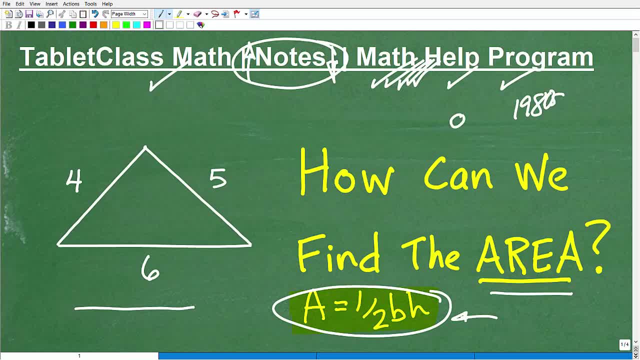 in school. what was I doing during math class? Well, I was talking to my friends and they were talking to me, so I wasn't the only one. I was quite distracted and my notes were like blank, And if there were anything on it, it was probably scribble scratch. Maybe I was just writing stuff. 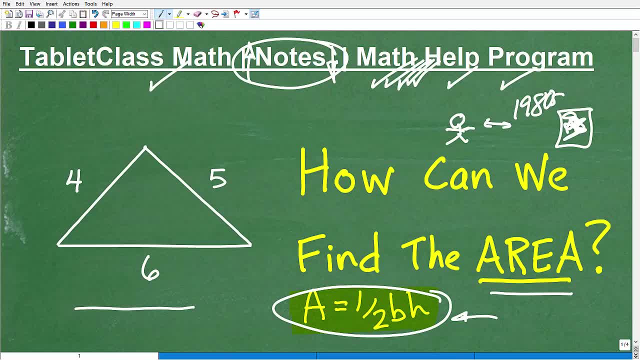 down to pretend, when the teacher was looking at me, that I was taking notes. But I was really jottering, I was just doing whatever. right? So you get it, And I'm not trying to pick on you if this is your situation, Because, as a teacher, when you observe a classroom, you see everything. 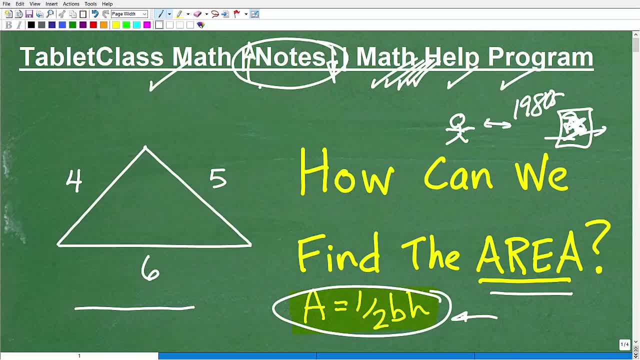 Okay. so just if, by the way too, it's just a little inside tip- If you're a student in that classroom, okay, and you think the teacher is not seeing what you're doing, you better think again, because teachers really see a lot more than you probably think And you observe activity. 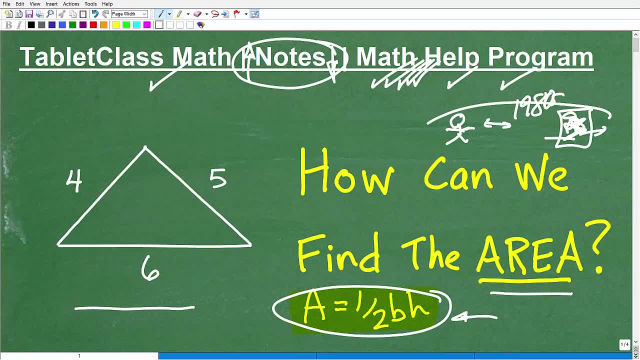 you see who's working, you see who's not, etc. etc. But anyways, I paid a price. that wasn't until later on, when I went to college, I actually learned how to become a good student. But the bottom line is this: okay, you have to take notes to remain focused. Focus is the key. okay, So focus. 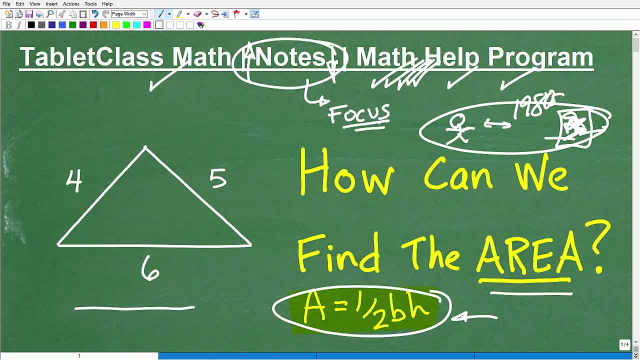 is the key to learning anything, And the only activity I know of that will keep you extremely focused- and you need extreme focus when you're learning mathematics- is note-taking. okay, All right, so in the meantime, as you're improving in your notes- because I'm pretty sure most of you 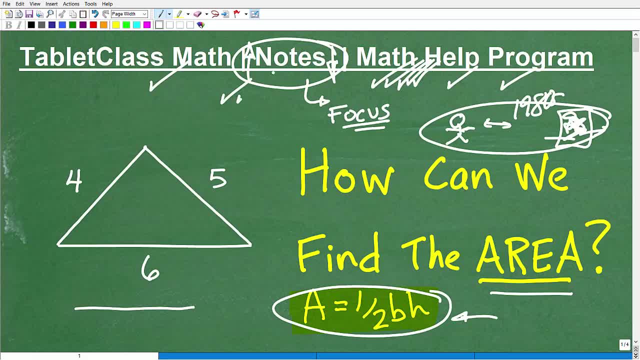 I offer detailed, comprehensive math notes to include pre-algebra, algebra 1,, geometry and algebra 2, and trigonometry. You can find links to those notes in the description of this video. Now let me just kind of say a little quick heads up here. I'm kind of fighting a little. 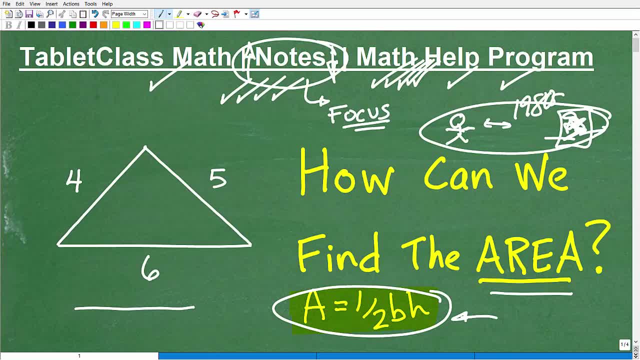 seasonal allergy. so if my voice breaks up, please forgive me. But guess what? That's not going to stop me from trying to help you learn mathematics. So let's continue on and figure out the area of this triangle Now. by the way, if you think you know what I'm talking about, 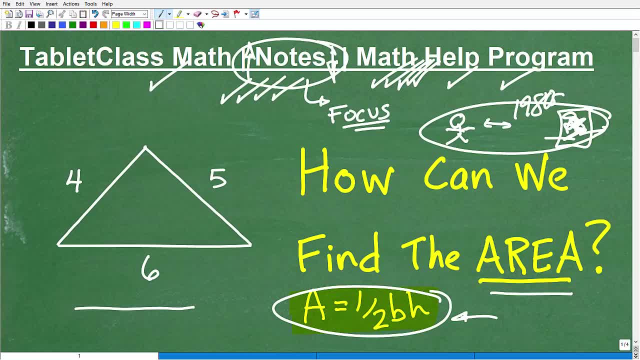 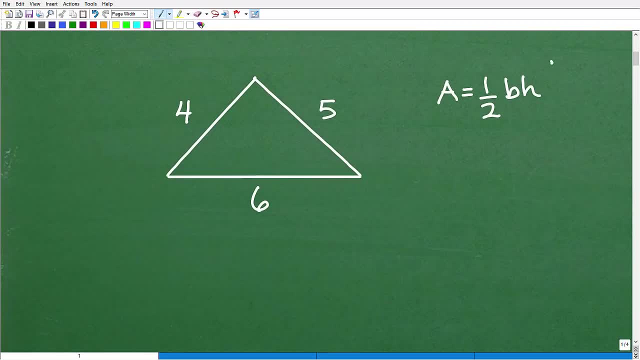 how to do this problem. go ahead and pause the video and do it, But let's get to it, okay. All right, so here is our triangle and here is our trusty formula: area equals one-half base times height. So again, if you were thinking, oh, I know how to find the area of a triangle, I use this: 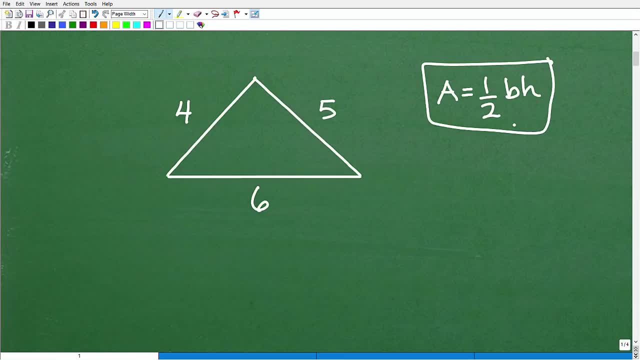 formula. The problem is with this particular formula. you need these two pieces of information, So you need the base. Now, any one of these these sides could be the base. If I kind of rotate the triangle and I don't want to kind of 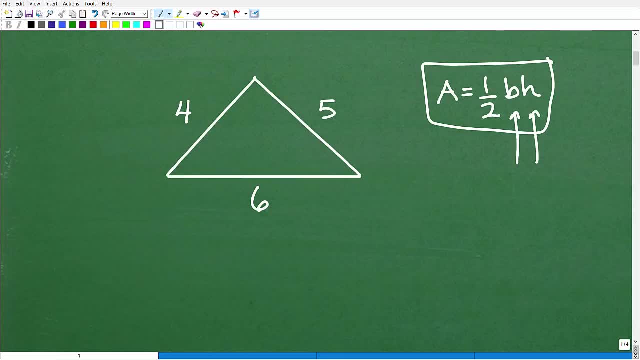 get too far into too many side topics here, but the four could be the base, the five could be the base, But let's just look at this triangle the way it's, kind of in its current form. So this right down here, let's consider that the base. So, okay, I have the base. So if this is the base, okay. 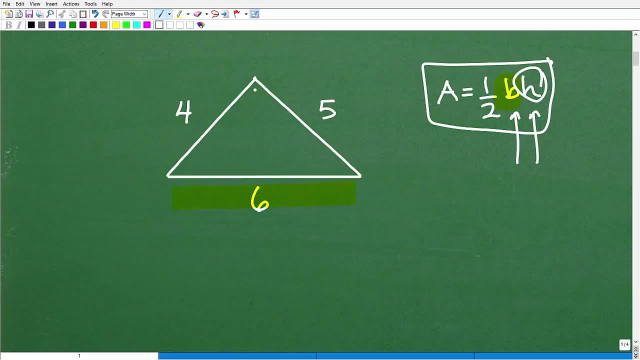 I need the height, okay. So what's the height? Well, the height is going to be from here to here, okay, So this is the height of the triangle. Well, I don't have the height, okay, And I need the height to use this formula. So how do I get this piece of information? How do I get? 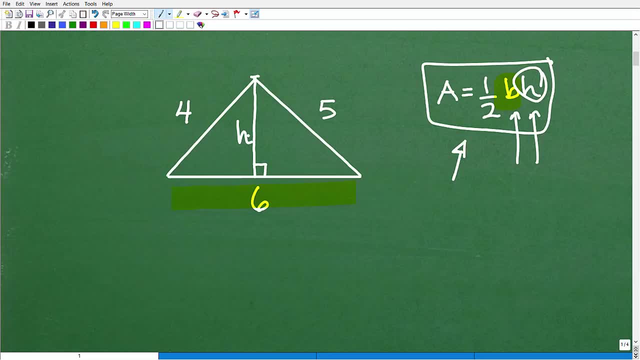 that. Well, you're going to need some additional mathematics. okay, There's some things you could use from geometry. We could actually find the angles using the law of sines, law of cosines, and this is kind of pretty sophisticated stuff. Again, you could use. 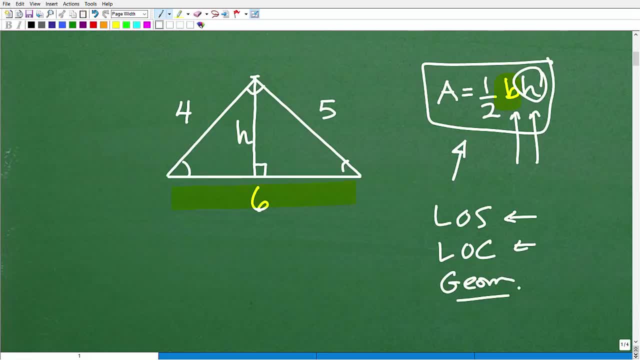 uh, some, uh, geometry, um, and properties of triangles, But what I'm going to share with you is an awesome formula. Just, you know something like this: This is a formula to calculate the area of a triangle. Well, guess what? There's another formula that we can use to find the. 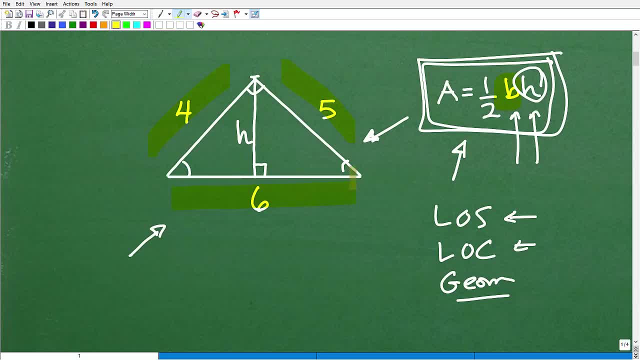 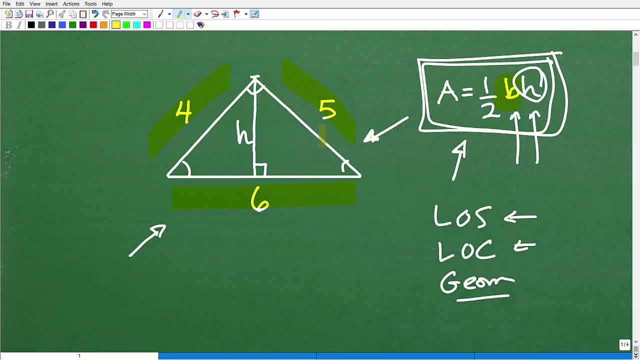 It's not obtuse or acute. Well, you could uh make the case for, uh, this maybe being an acute triangle, But, uh, if you don't know what I'm talking about, don't worry. This is stuff that. 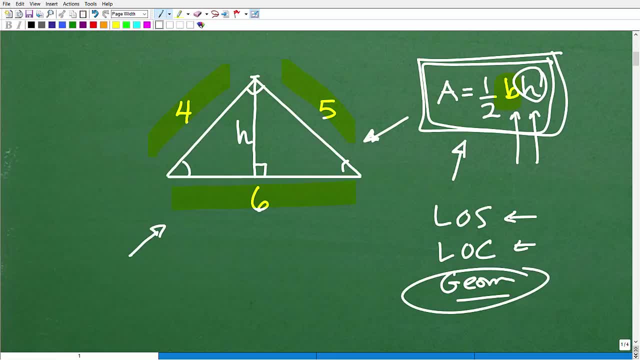 you learn in geometry. The bottom line is we have a triangle and we have the three sides of a triangle and we want to find the area. Okay, So, whether it's a right triangle, uh uh, obtuse or acute, uh, we can use this formula. So let me get to that formula right now, And then we'll go ahead. 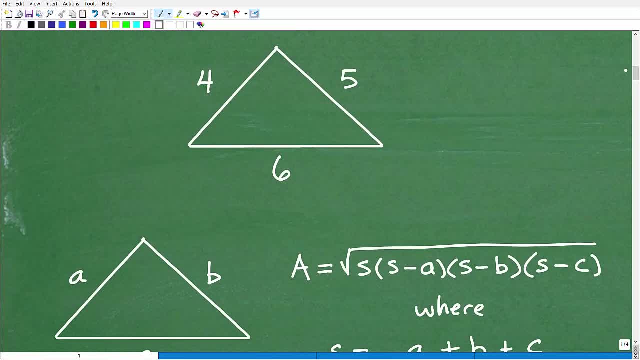 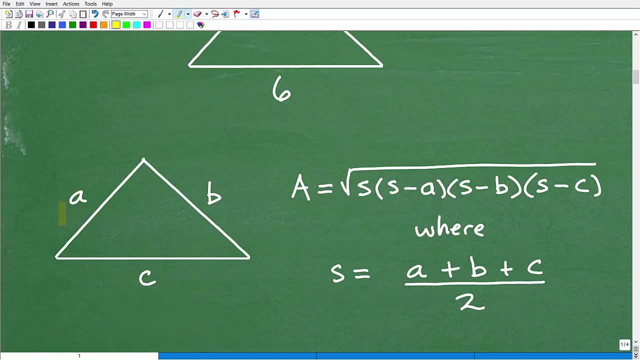 and calculate, uh, the area. Okay, So here is our triangle and here is the formula. Okay, So let's take a look at this formula. So here is a triangle with sides A, B and C And, uh, here is the. 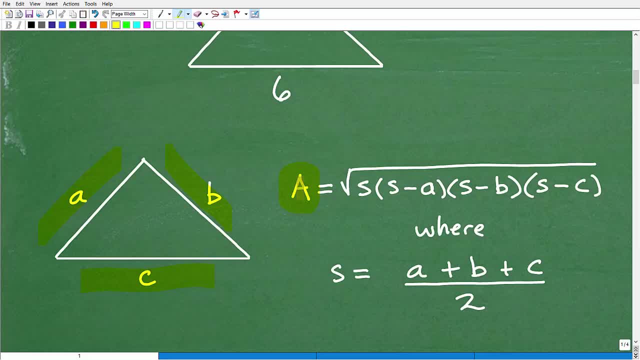 formula for the area. However, let's not look at this, uh, right now. Let's look at this part. We need this S and S, Okay, We need S to use this, Okay, So let's just look at what S is. So S is. 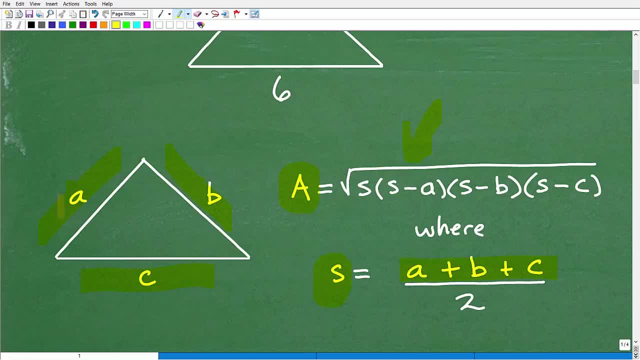 uh, we're going to add a triangle. We're going to add a triangle. We're going to add a triangle. We're going to add up A, B and C. Okay, We're going to add up the sides of the triangle and. 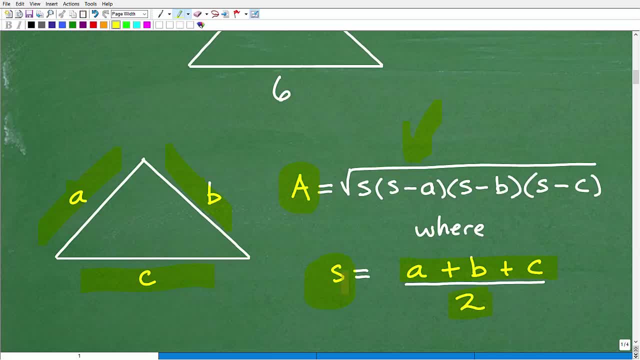 divide by two. So when we calculate this out, this is going to be this number: S. Okay. So now, now that we have this S, we can find the area of this triangle by taking the square root of all of these things right here. We're going to take S. okay, whatever that number is, excuse me, and 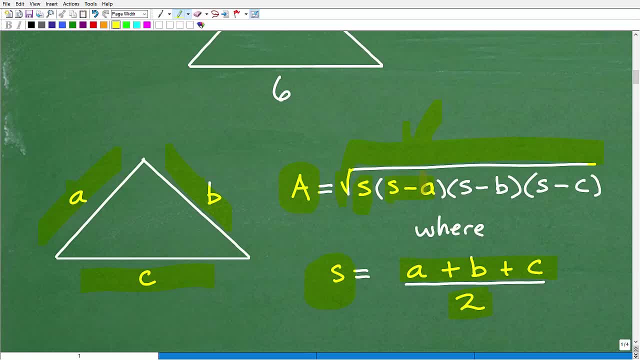 we're going to multiply it by S minus A, Okay. So whatever this value is right here, we're going to subtract this length right there, Okay, And then we're going to continue to do the same. We'll plug in our S right there, and then we'll subtract B and then S right there, and we'll subtract uh. 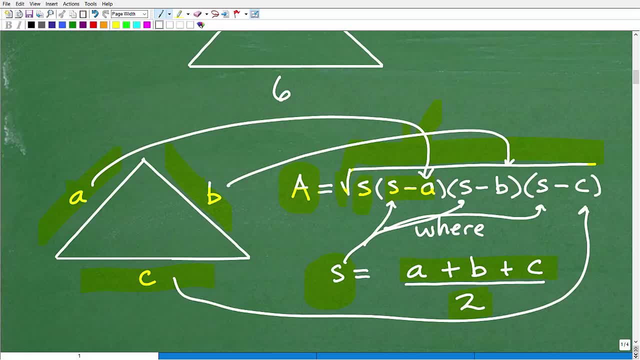 C. Okay, So we just got to basically follow this uh formula very specifically, Okay, By first calculating S, then plugging in the respective uh values for these variables and uh doing the number crunching, and then we can find the area. Uh, obviously, uh having the number crunching. 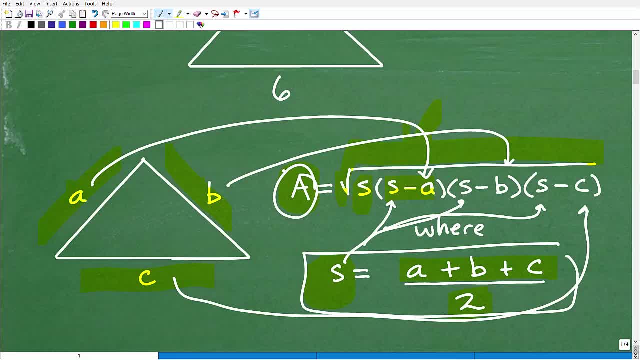 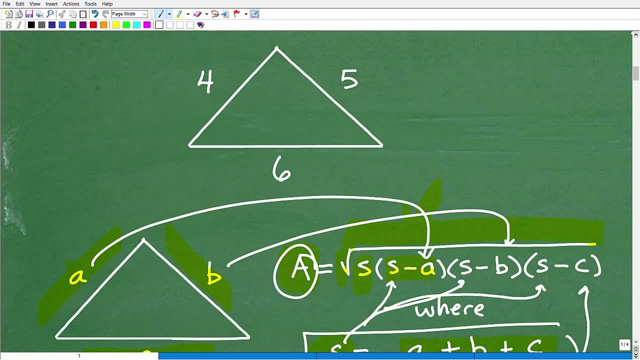 having a calculator would be very useful for this exercise. Okay, Now, if you think you got the idea and you're like, okay, now I can, uh, uh, do this problem. So here we have four, five and six. 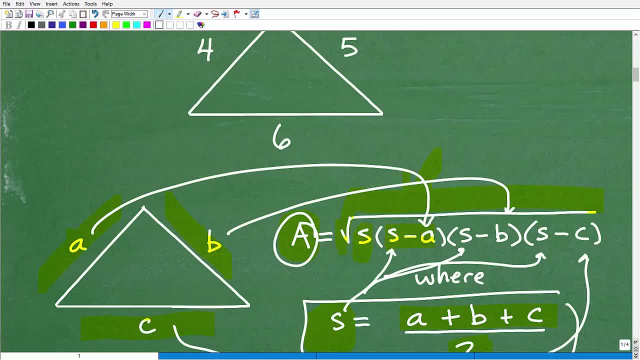 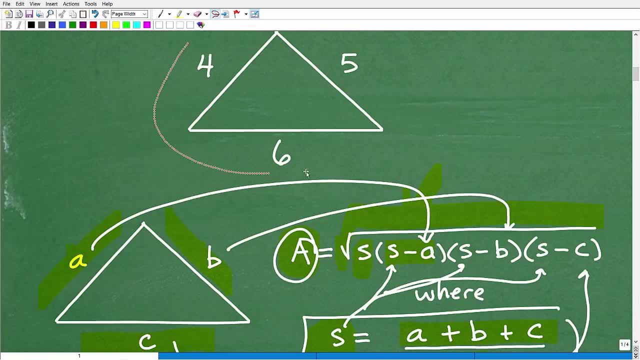 Now that is our triangle, Okay, And here I'm kind of trying to put it in uh- where you can kind of still see. well, you know, let me just move it here. So I want to give you an opportunity. 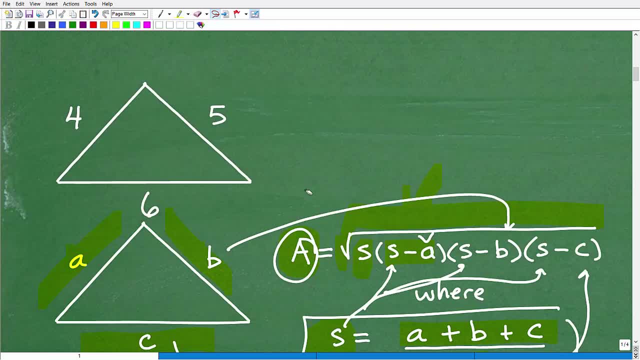 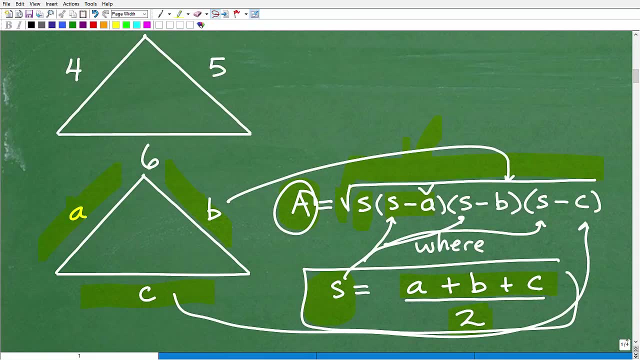 to actually do this problem before I do it, because really it's just an application of following a uh formula. Okay, And you need to be able to follow formulas in mathematics. So go ahead and pause the video and give it a whirl and see what you come up with. Don't be shy about using 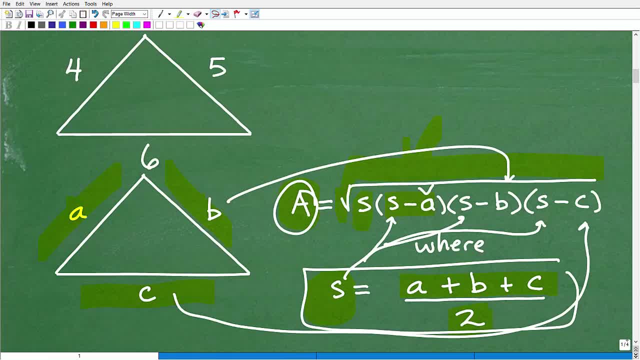 a calculator, um, to assist you. You're definitely going to need one. but uh, you know, plug in all the values, do all the number crunching And uh, if you don't want to see the answer, go ahead. and. 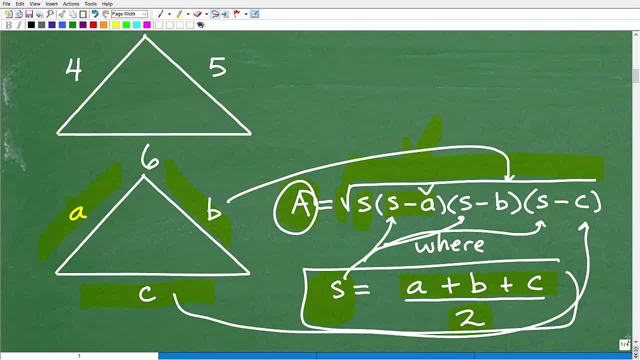 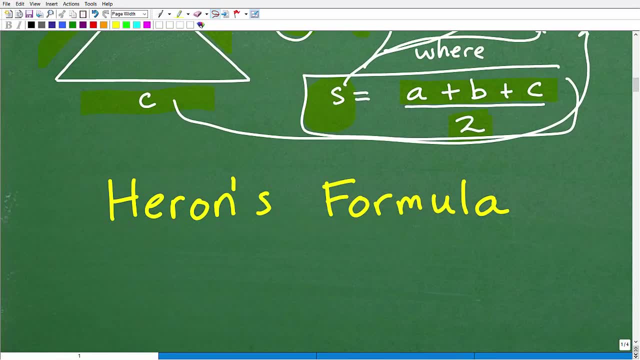 put it on pause, because I'm going to go ahead and show you the solution right now. Okay, Here we go. By the way, I failed to mention this is probably you know. I was really gonna- uh, you know- make a mistake here by not mentioning 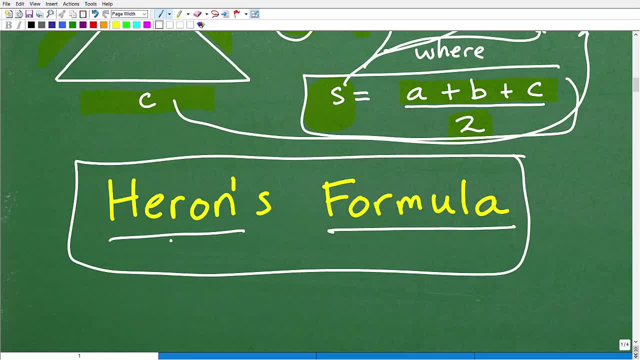 what this formula is. Okay, This is uh Heron's formula. Uh, it's kind of pronounced different ways, but anyways, uh, this is how it's spelled. uh, Heron's formula. Excuse me, Boy, it's that. 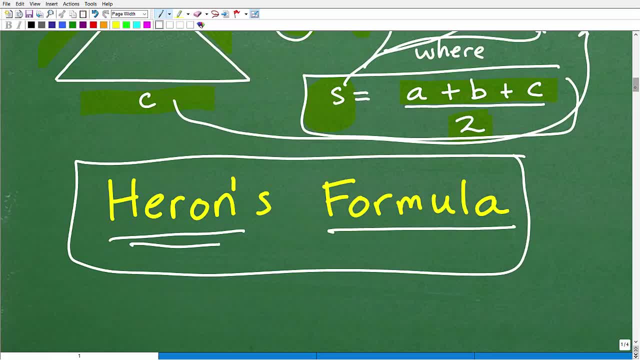 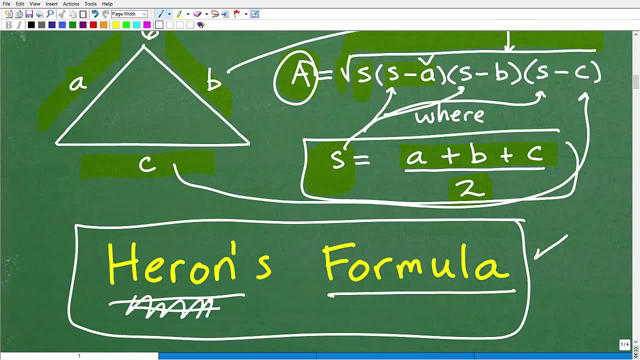 time of year when I'm fighting these allergies, but uh, so forgive me when my voice breaks up, But anyways, this is the name of this formula: Super, uh, famous. This guy was just like a superhero in geometry. So many uh uh, huge uh formulas or names uh behind the formulas. 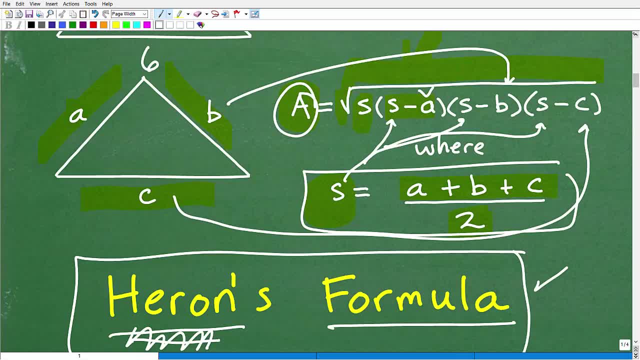 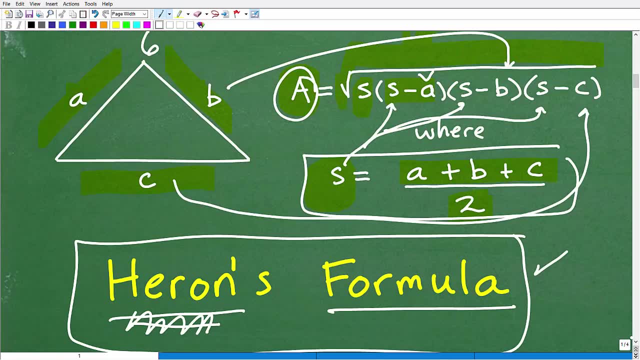 like the Pythagorean theorem was named after Pythagoras, which was, like this, just awesome, uh, mathematician, I mean, these, these are- and these are guys too- that lived, like you know, thousands of years ago. So it's pretty crazy, you know, uh, but people were able to figure out. 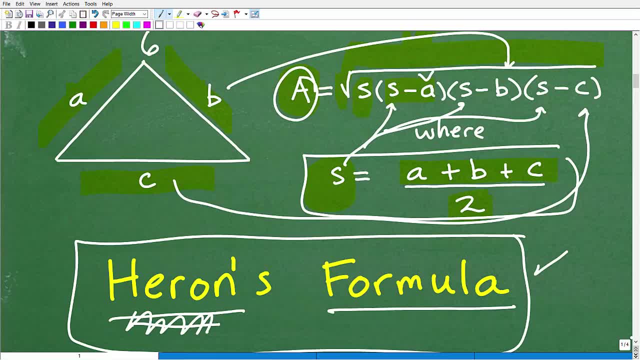 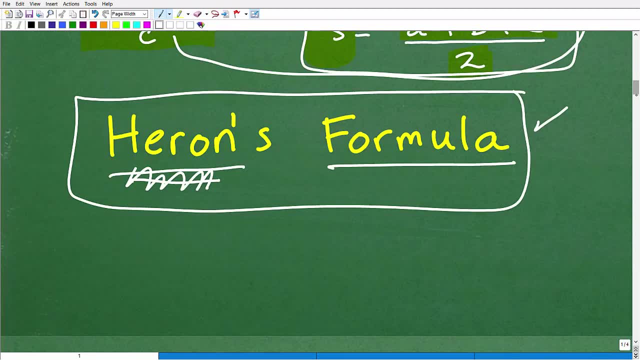 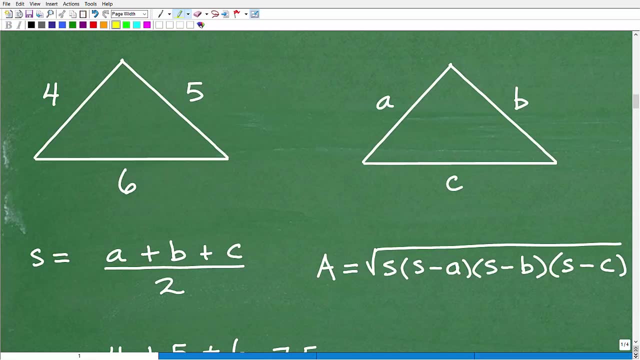 you know all this time ago, but, uh, and we use it today, right? So this is the name of the formula, and this is the formula, And now let's get to it. Okay, All right. So again, this is, uh, really an application in number crunching. So here is our 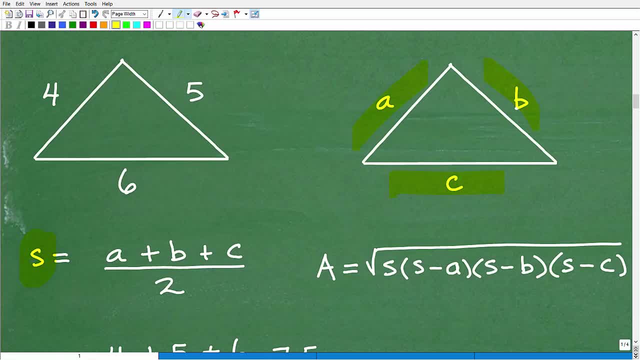 side ABC, and we're going to start off by first finding uh S. So we're going to, uh, uh, add up each of these sides, uh four, five and six right here, and divide by two. So let's go ahead and do. 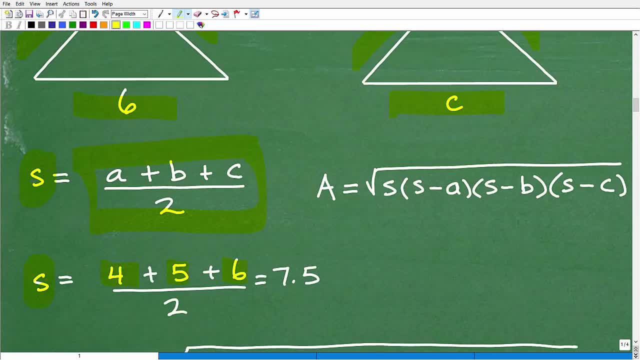 that now. So S is going to be four plus five plus six, And then when we divide that by two, of course, that by two is 7.5.. So we're going to plug in our 7.5 here, here, here and here, And then we'll. 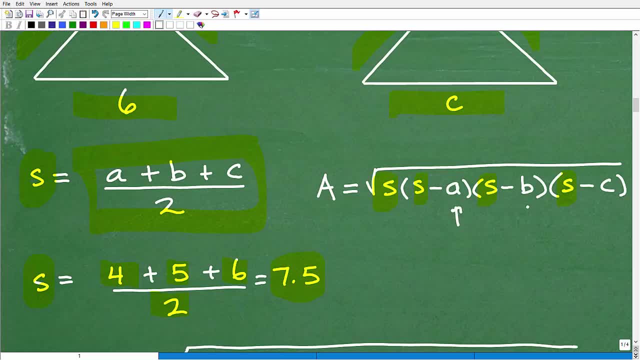 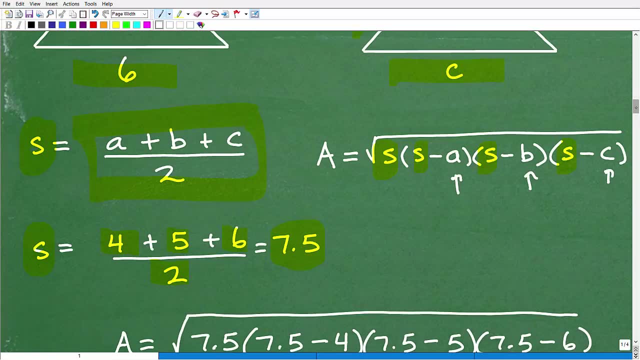 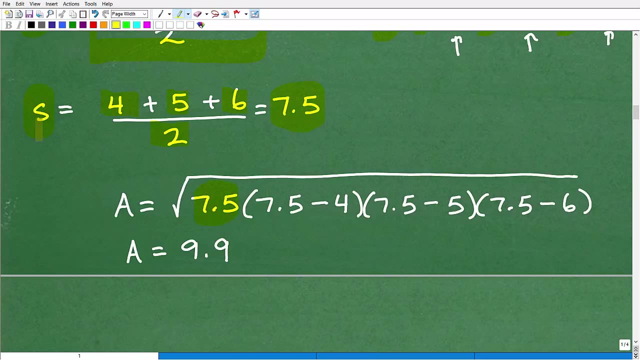 plug in the respective uh sides of the triangle in these spots, And then we'll do all the number crunching. So let's go ahead and take a look at what that looks like. And here it is. I kind of spared you all the number crunching. So this is S right. So S is 7.5. And now we have 7.5 or S minus. 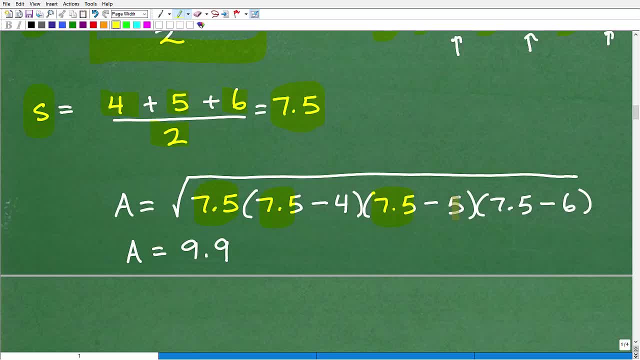 the triangle, which is four, And then we have 7.5 minus the other leg, which is five, and 7.5 minus six. Now notice that this is, uh, in parentheses, grouping symbols, So you do have to calculate this. 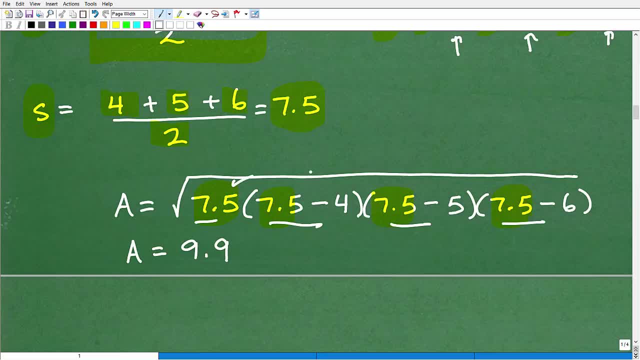 out, uh, these individual numbers, and then multiply this times, this, uh, the result of that and the result of this and the result of this. So you're going to have this product. Once you have that, then you take the square root and you're going to get 9.9.. Okay, And that is the area Of course. 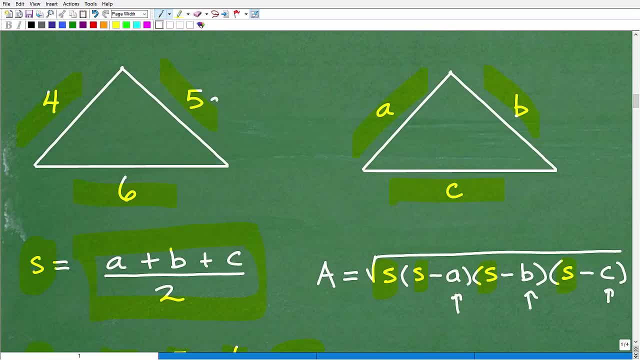 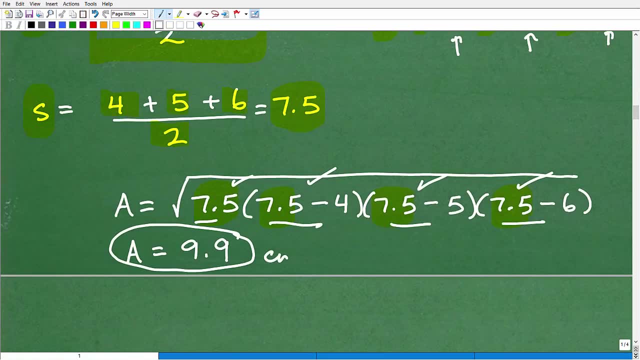 we don't have any uh units of measure here. In other words, if this was like centimeters, uh, for example, uh, our area would be in uh centimeters squared, So just keep that in mind. But in this case, uh, 9.9 is the answer. 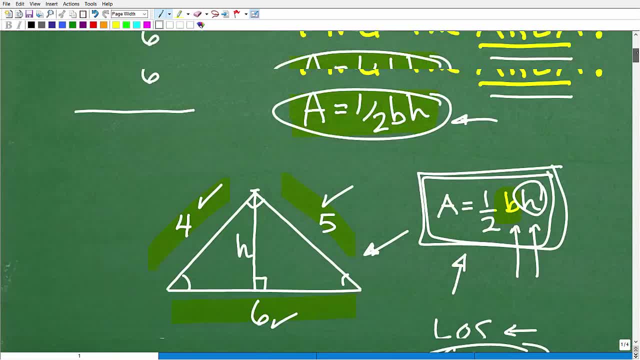 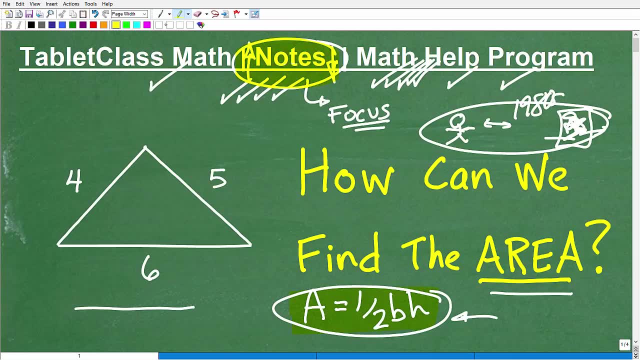 And there you go. Okay, This is how you find the area of problems like this. This is a great formula, And it's something that I would definitely suggest you put into your notes. Okay, Because a problem like this can very well come up again in your future. 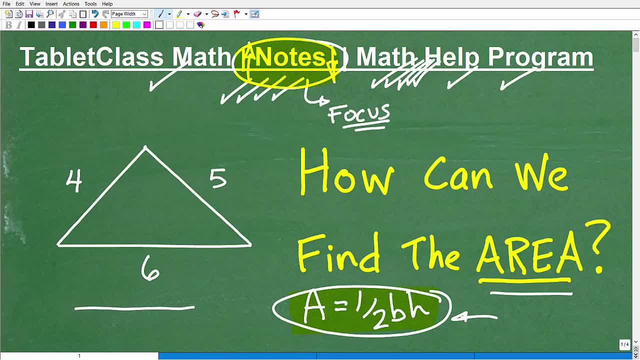 You never know. Okay, All right. So if, uh, in some way you kind of liked this video, you enjoyed it and you're like, oh, I learned something, Well then please consider smashing that like button. That definitely helps me out. And, uh, if you're new to my YouTube channel, please consider. 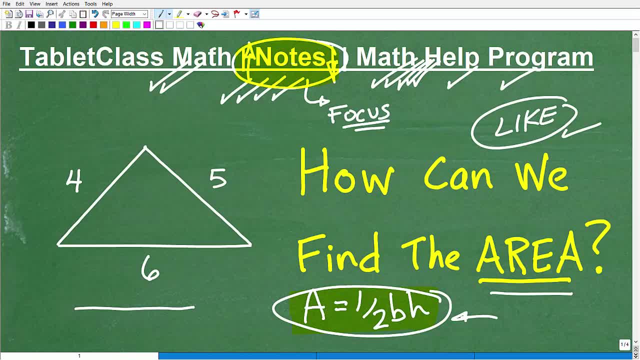 subscribing. I've been on YouTube for well over 10 years. I have a lot of videos, maybe like over a thousand, I don't even count. Uh, what I do is I really explore how I can help those out there learning mathematics. on my channel, By the way, you'll find various playlists organized from basic. 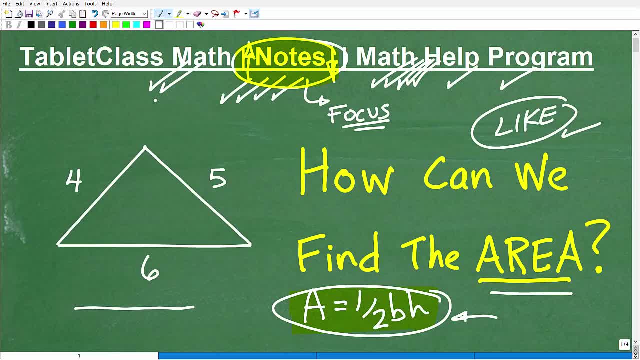 advanced mathematics. Um, and my goal is to really teach math in a clear and understandable way. Nobody should be failing math these days. Okay, Um, if you're struggling in math, uh, again, start with your note-taking is probably, and you've got to do your part as well, right You? 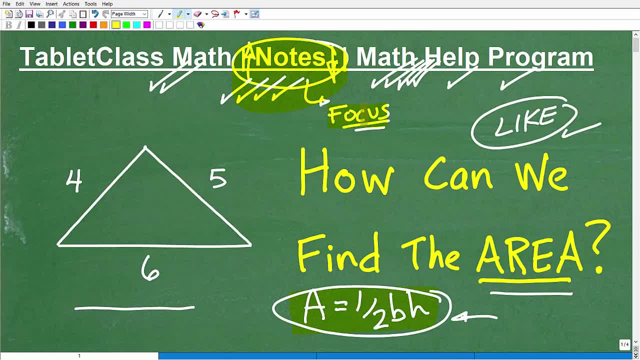 can't just be blaming it on your teacher. I know a lot of people- including myself, I'm sure- I was like: ah, my teacher is terrible. Well, you know, your teacher can't take your notes for you. You got to do your part, Okay, So if you're working hard and you're talking to your teacher, getting 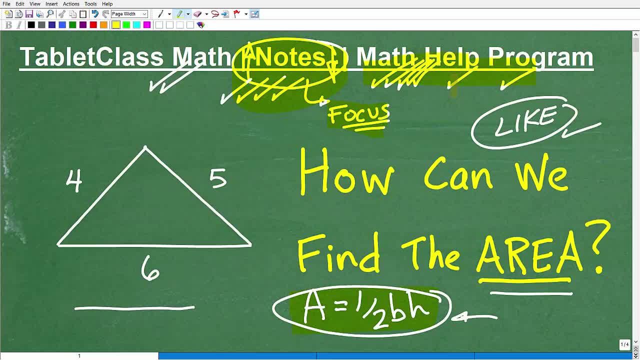 extra help, even if you're that's not enough, then there's a tons of uh resources. uh today that uh you know you can, you're going to have to take the initiative to help yourself. So, if you like my 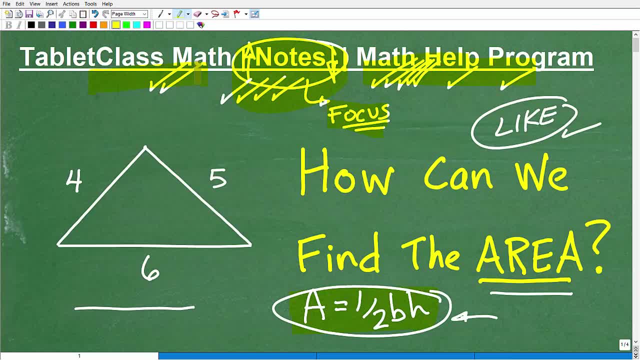 teaching style. there's a ton of uh stuff on my uh channel and I'm posting new material all the time, but, uh, my best math help will be within my math help program. Okay, So, with that being said,